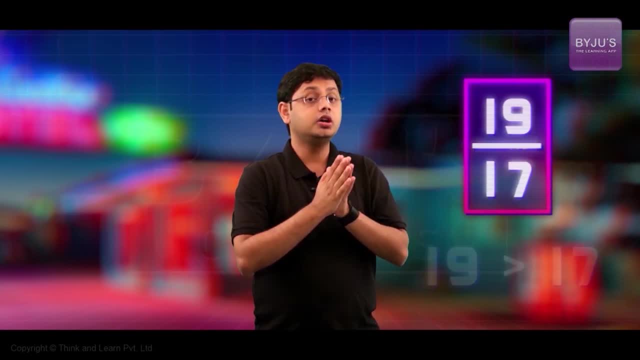 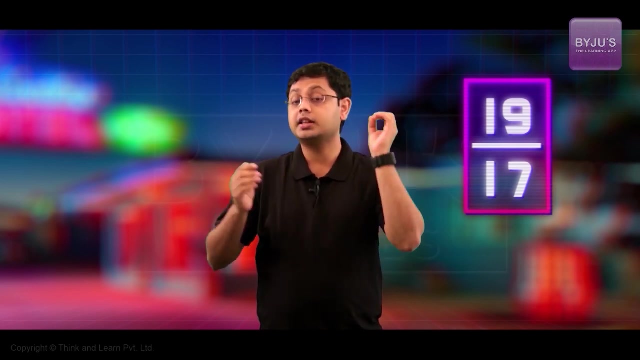 is actually bigger than the whole right. So this certainly does not represent proper fractions. So what do we call them? It does not even look like a proper fraction. It looks improper, right? Well, guess what? That's exactly the name given to such type of fractions: It's called improper. 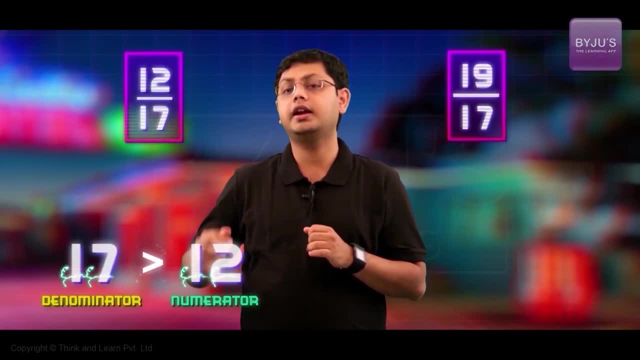 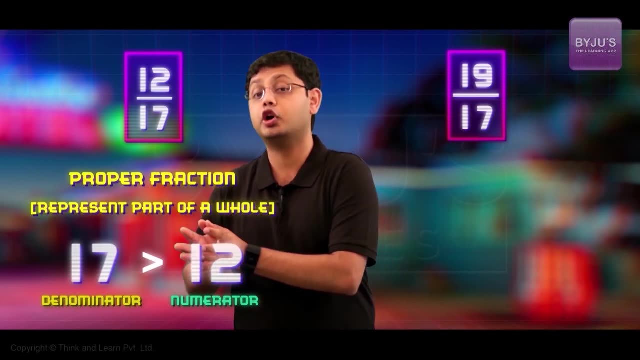 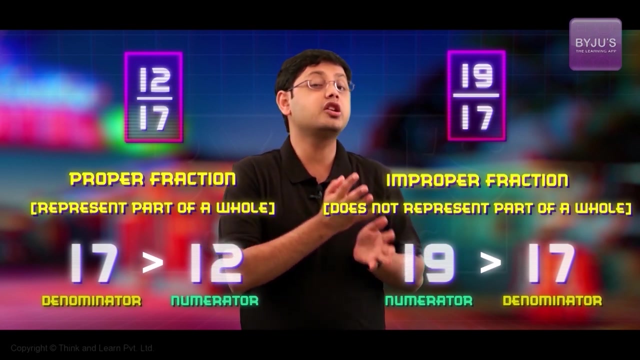 fraction. The fractions with denominator greater than the numerator, like you already know, are called proper Improper fractions because they represent part of a whole, Whereas fractions where numerator is greater than the denominator are not representing parts of the whole or the parts are bigger than. 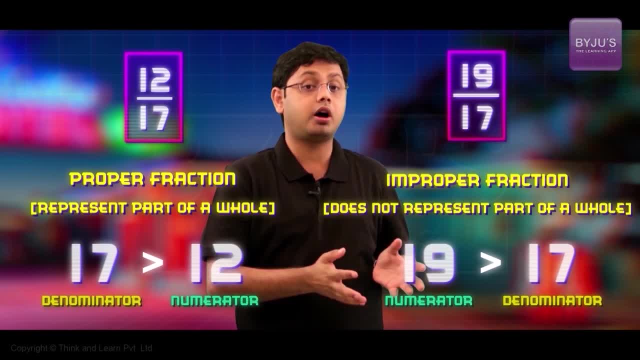 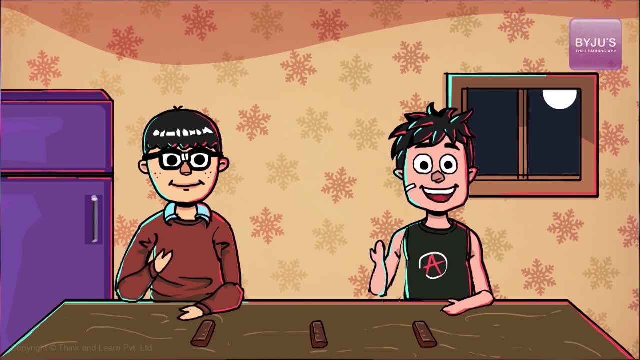 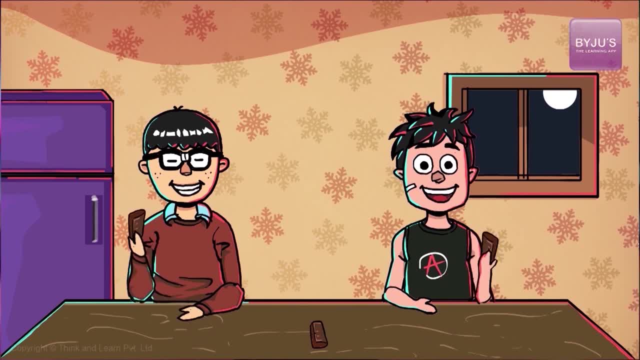 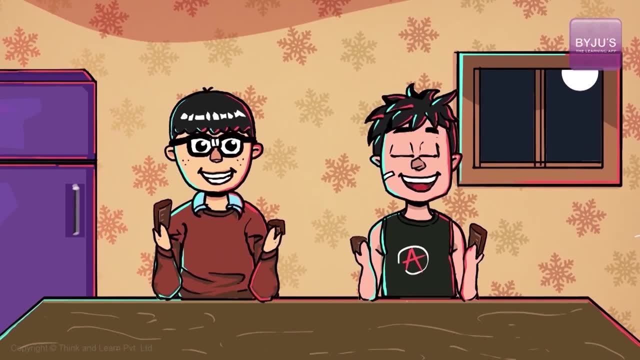 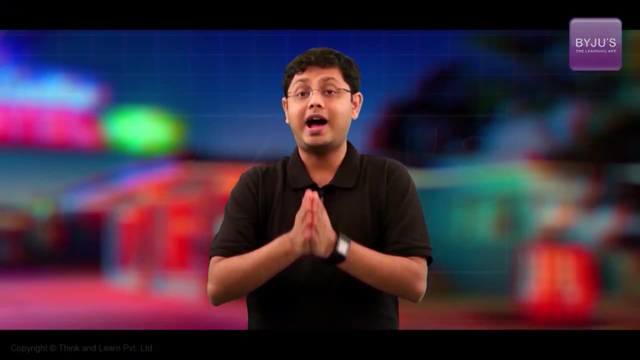 parts. right, You would each take one whole chocolate and divide the third chocolate into half and share it between you. So basically, you and your friend's share of chocolate will be one and a half. Now, what will that value be, Arjun, can you help me with that? 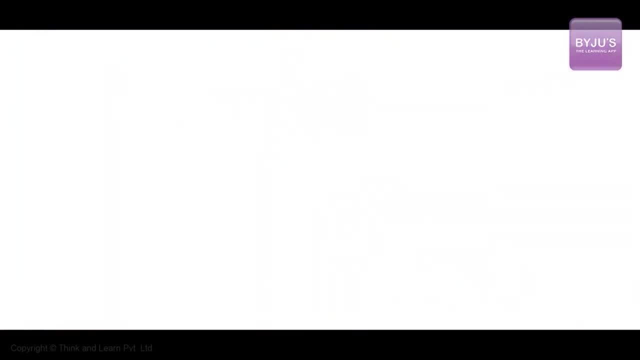 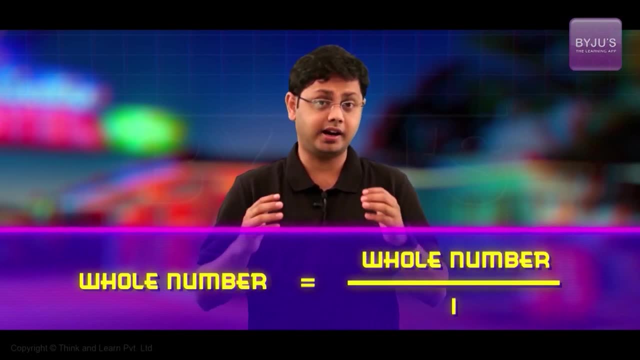 How do I add a whole number and a fraction? Well, I can write any whole number and write it as a fraction by dividing it by two parts. So I can write any whole number and write it as a fraction by dividing it by one right, Because any number divided by one will give that number itself. So 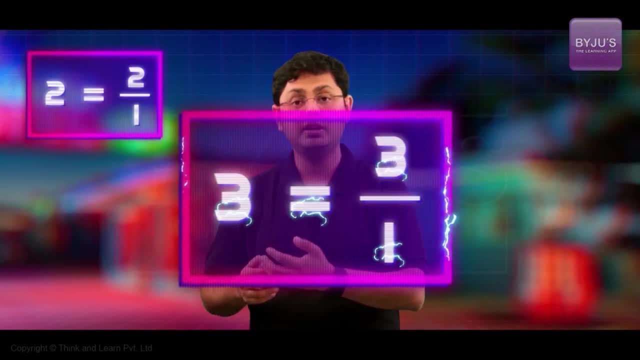 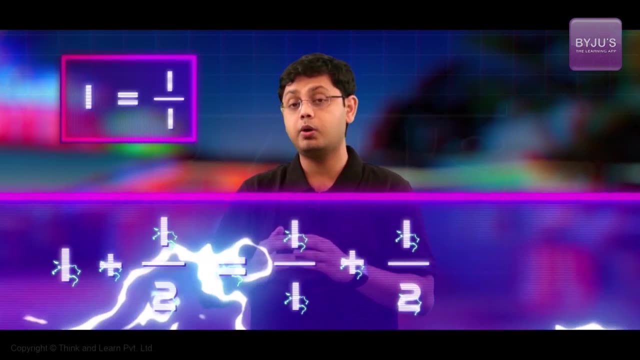 two can be written as a fraction as two by one. Three can be written as three by one. Five can be written as five by one, And in this case it happens to be one. Therefore, I can write it as one by one and I have to add a half to it. Therefore, the problem changes to one by one. 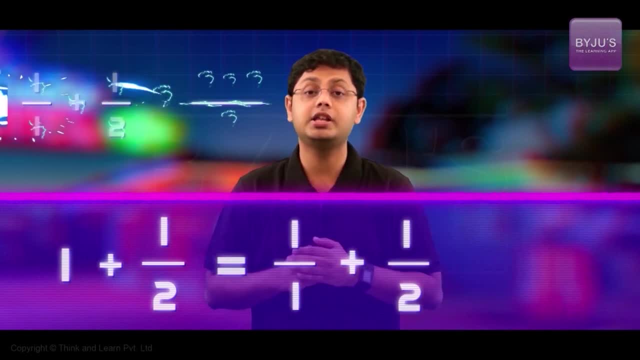 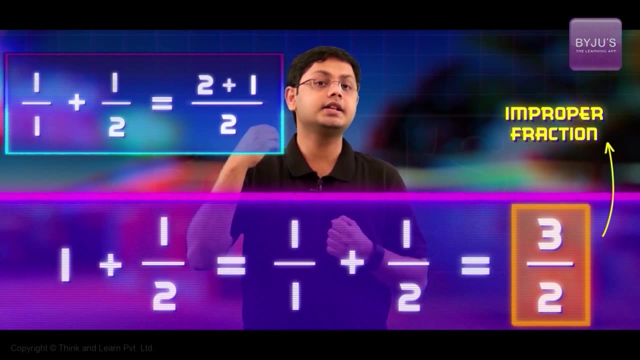 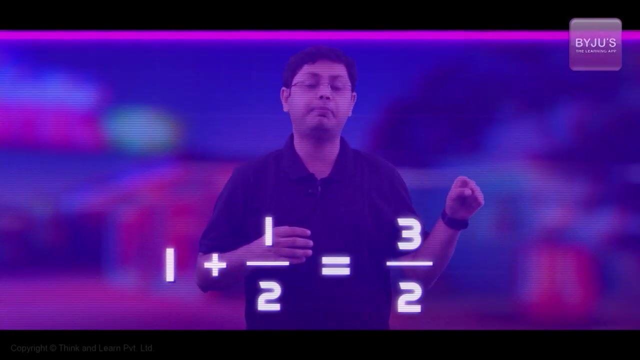 plus one by two. Now you can continue with the addition of unlike fractions, like what we solved before. Do you see that this is an improper fraction, as three is greater than two? So you saw what we did above, right, We added a whole part one chocolate.